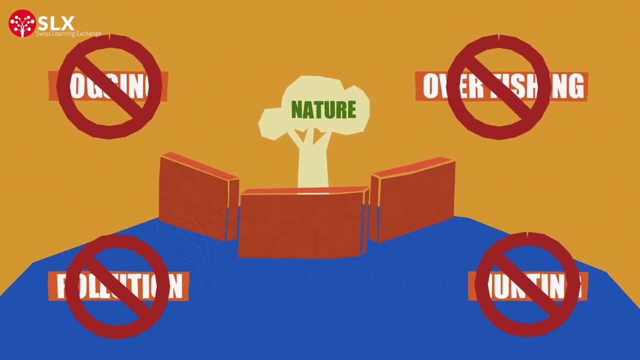 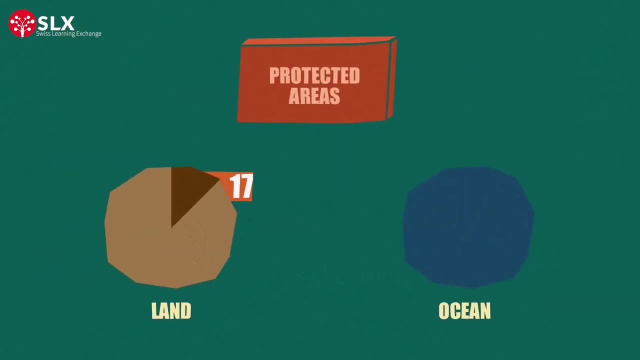 by limiting or banning these activities. The IUCN defines such spaces as protected areas. Today, nearly 17 percent of land and 7 percent of auchi are classified as protected areas. Besides conserving nature, there are other benefits these protected areas provide. A report published by CBD shows. 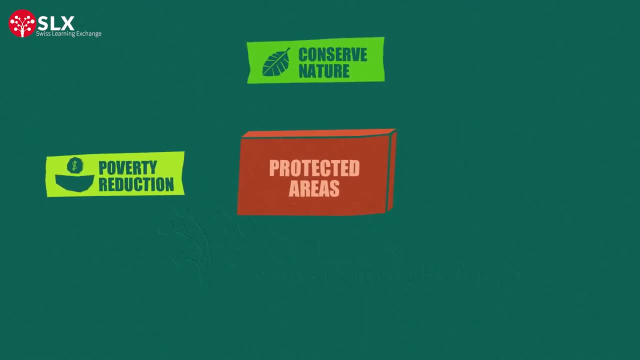 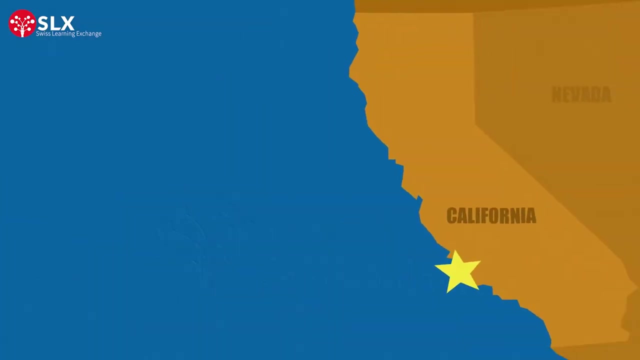 that protected areas can help with poverty reduction, provide clean drinking water, improve human well-being, promote ecotourism and, most importantly, preserve and strengthen ecosystem services. Researchers in Southern California revealed that establishing marine protected areas reduced fishing by 35%. 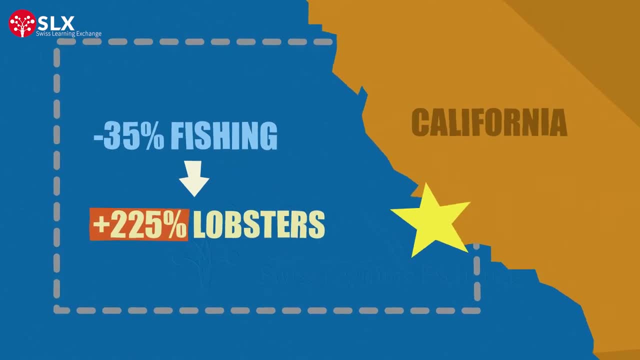 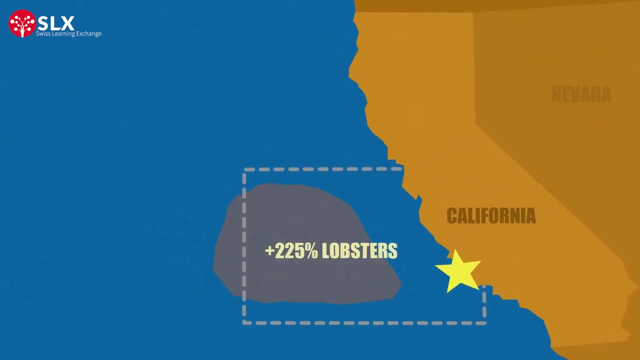 and yielded a 225% increase in the total catch of spiny lobsters after six years. due to an increase in spiny lobster density and biomass, This increase in lobster abundance spilled over to areas surrounding the protected area, whose people then also benefited from having more lobsters to fish In the 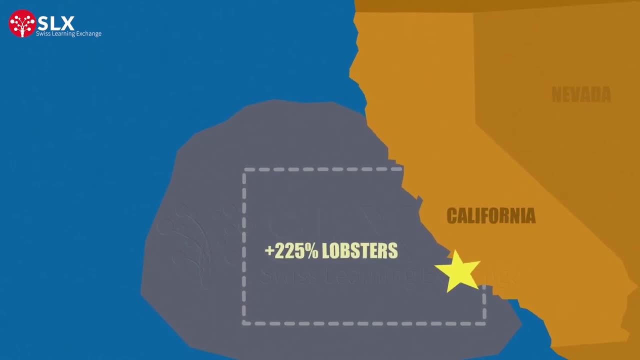 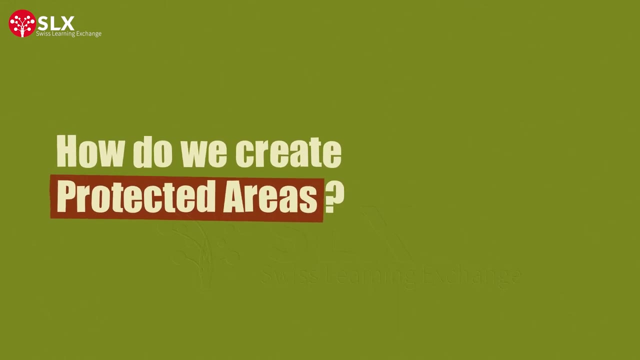 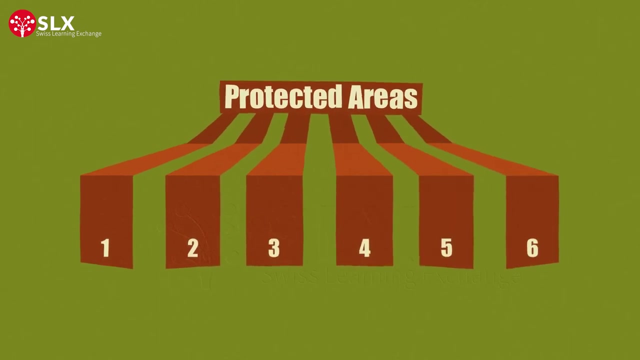 end. if done correctly, protected areas can benefit both nature and humans. The first step is to put a protected area in one of six categories. These categories are international standards defined by the IUCN, each with its own goals and protection criteria. Category one: areas have large intact natural. 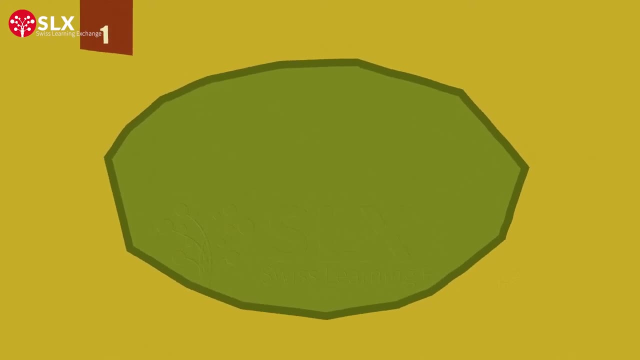 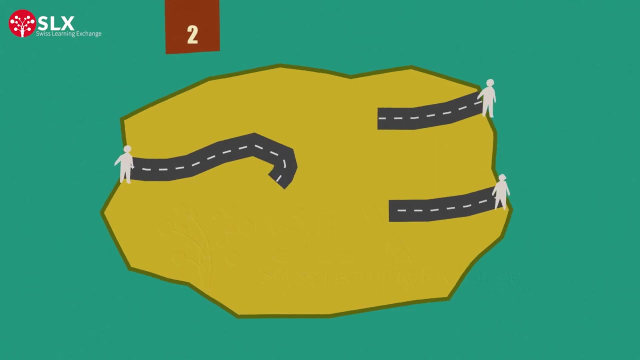 spaces where only special access, research and conservation work is allowed and human infrastructure like roads and electric lines is absent. Category two areas allow more human interaction, like recreation and tourism, to promote education and the local economy. They often have roads and visiting sites built. 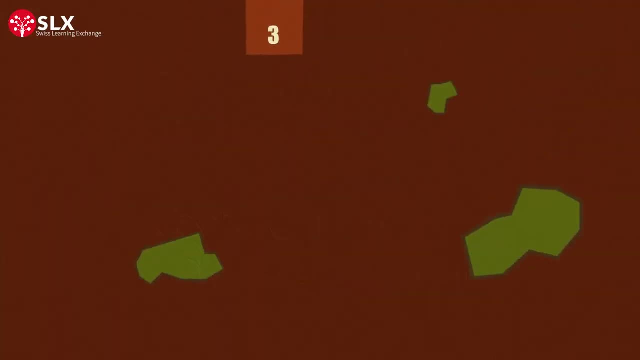 within them. Category three areas are like category two, but they are much smaller in size. Rather than conserving the entire ecosystem, they protect natural features considered significant, such as caves, mounts and waterfalls. Category four is similar to category three, but instead of 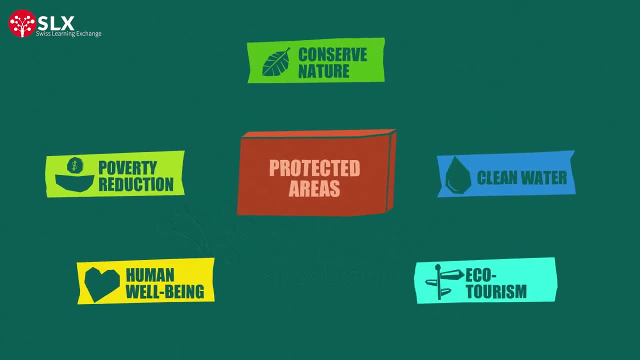 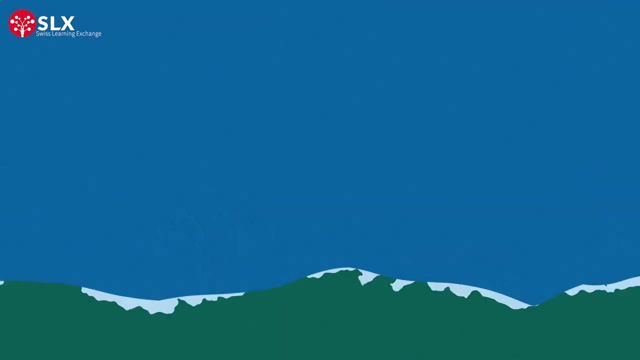 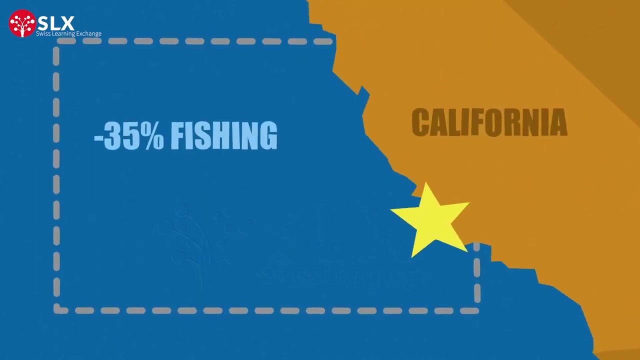 water, improve human well-being, promote ecotourism and, most importantly, preserve and strengthen ecosystem services. Researchers in Southern California revealed that establishing marine protected areas reduced fishing by 35% and yielded a 225% increase in the total catch of spiny lobsters after six. 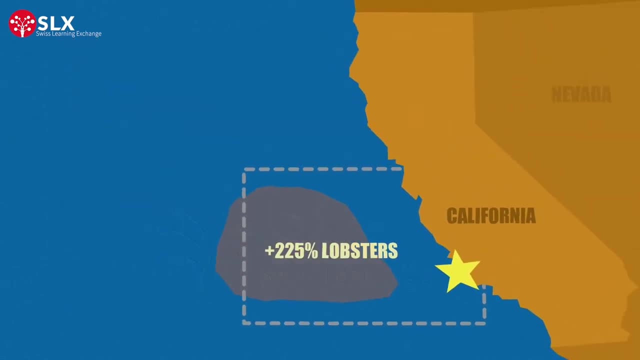 years, due to an increase in spiny lobster density and biomass. This increase in lobster abundance spilled over to areas surrounding the protected area, whose people then also benefited from having more lobsters to fish. In the end, if done correctly, protected areas can benefit both nature and humans. 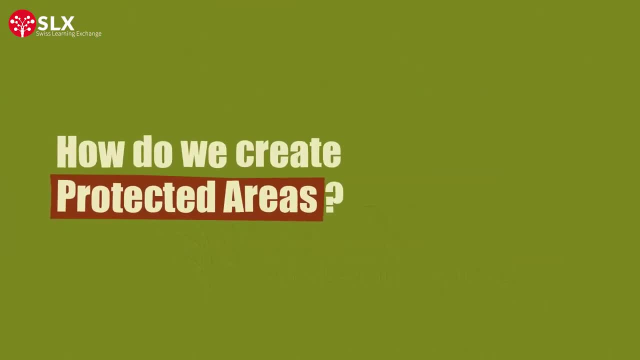 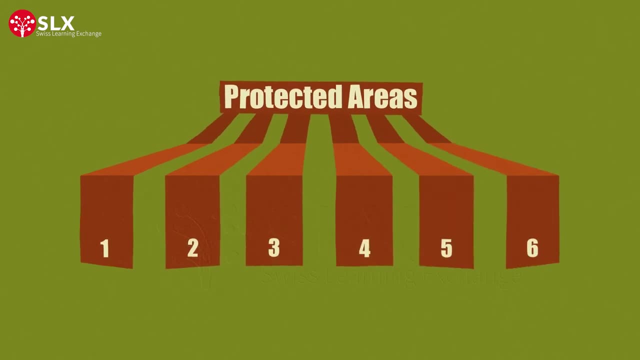 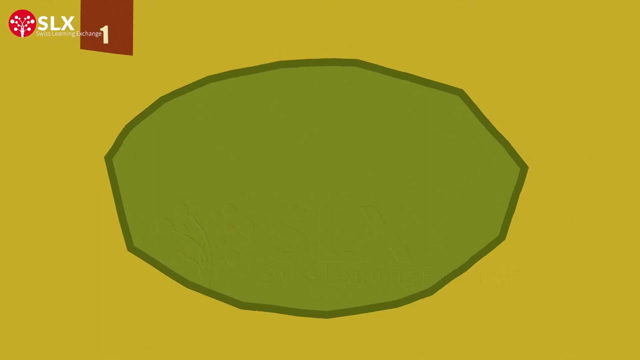 The first step is to put a protected area in one of six categories. These categories are international standards defined by the IUCN, each with its own goals and protection criteria. Category 1 areas have large intact natural spaces where only special access, research and conservation work is allowed and human infrastructure like roads and 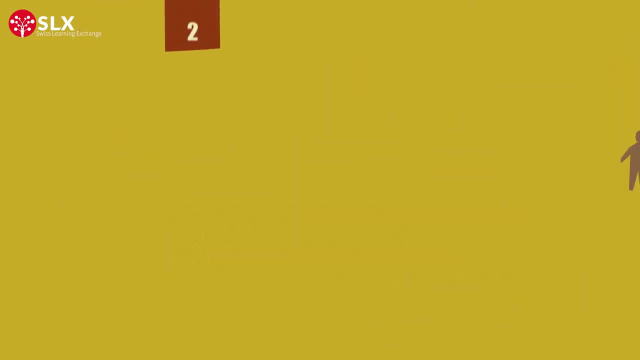 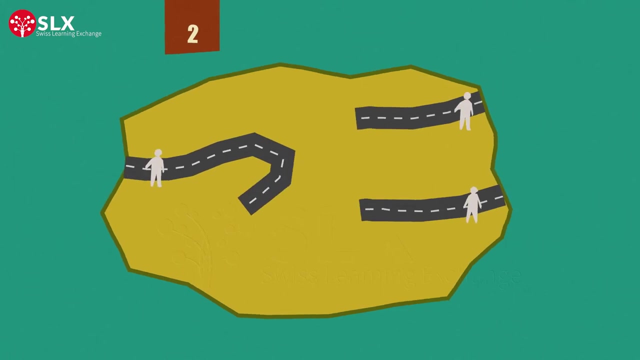 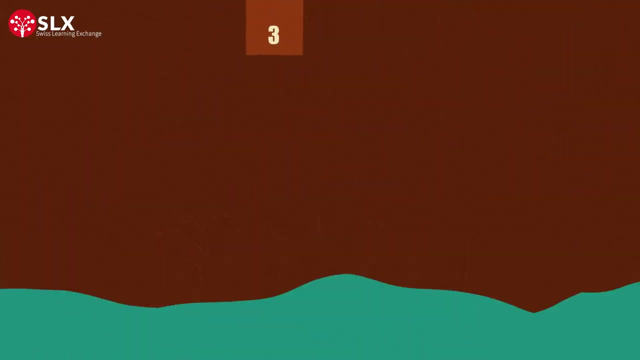 electric lines is absent. Category 2 areas allow more human interaction, like recreation and tourism, to promote education and the local economy. They often have roads and visiting sites built within them. Category 3 areas are like category 2, but they are much smaller in size. Rather than conserving, 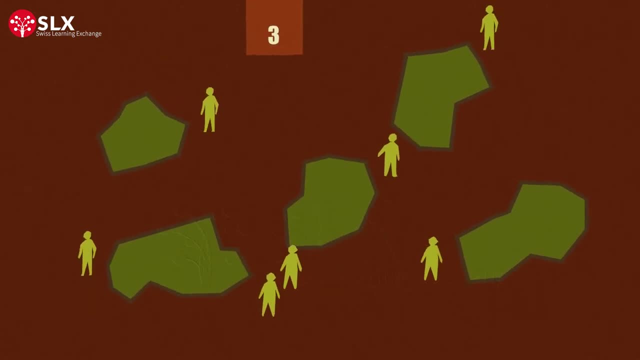 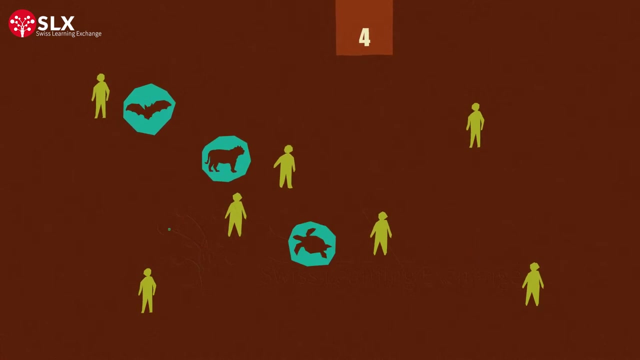 the entire ecosystem. They protect natural features considered significant, such as caves, mounts and waterfalls. Category 4 is similar to Category 3, but instead of protecting a natural feature, they protect a specific habitat or species. For example, the National Shambhal Sanctuary in central India focuses on conserving river dolphins. 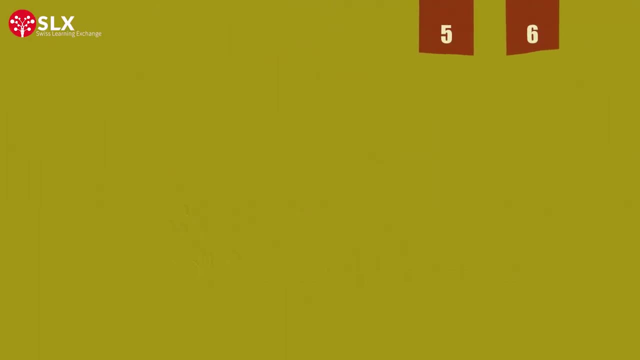 Categories 5 and 6 are areas that provide the least amount of protection. They are often larger than Category 3 and 4 areas and allow even more human interaction. Category 6 is unique because it allows local people to sustainably extract natural resources. 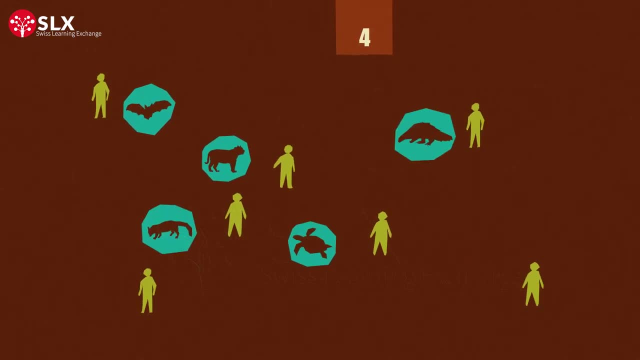 protecting a natural feature. they protect a specific habitat or species. For example, the National Shambhal Sanctuary in central India focuses on conserving river dolphins. Categories five and six are areas that are protected by the IUCN and the IUCN's 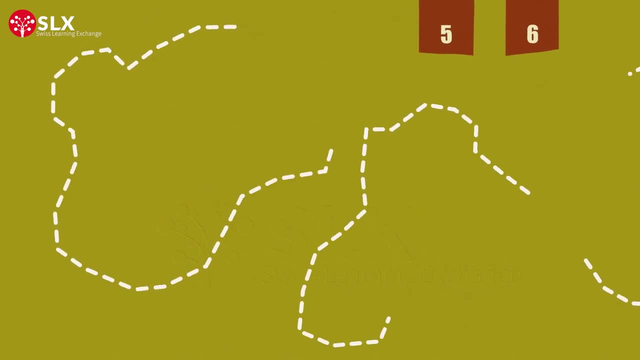 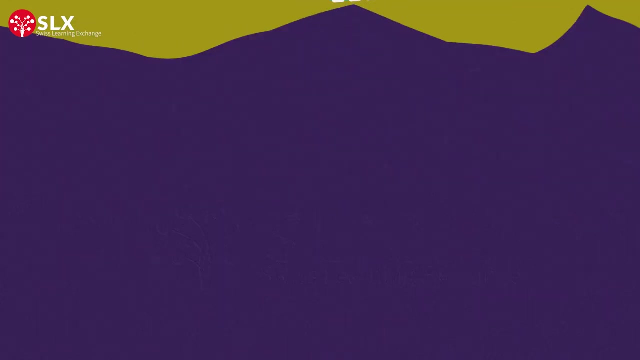 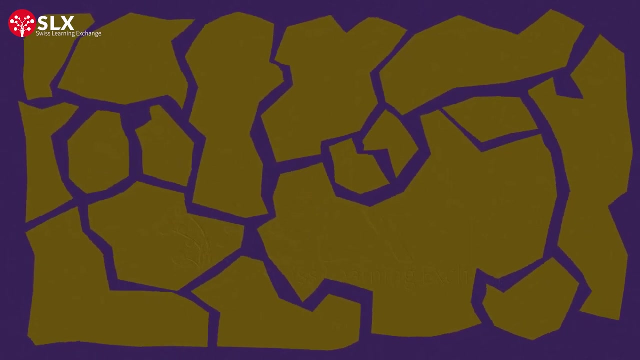 National Shambhal Sanctuary provides the least amount of protection. They are often larger than category three and four areas and allow even more human interaction. Category six is unique because it allows local people to sustainably extract natural resources. After categorization comes prioritization. Which area to conserve first To prioritize? 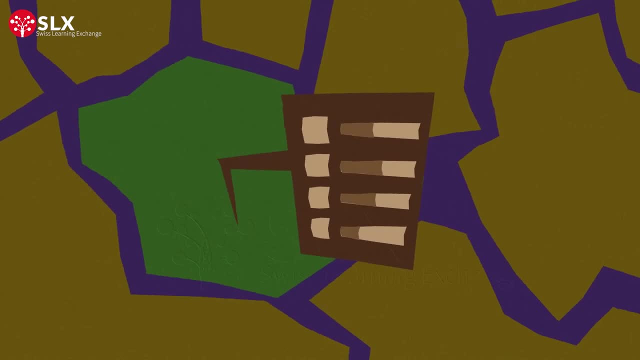 an area to protect, you need to first identify the area to be protected. If you are not able to protect an area, you must first understand the benefits it provides and assess how vulnerable or irreplaceable the life in the area is. Then we must assess the costs and benefits. 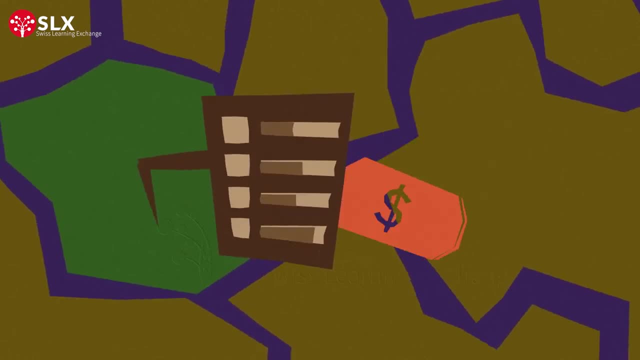 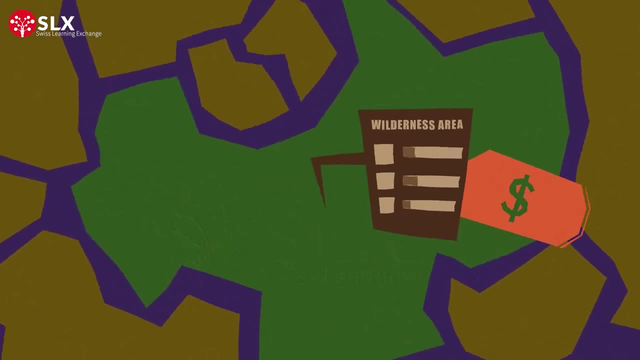 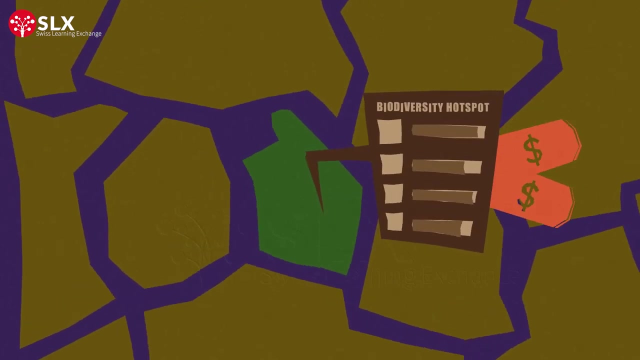 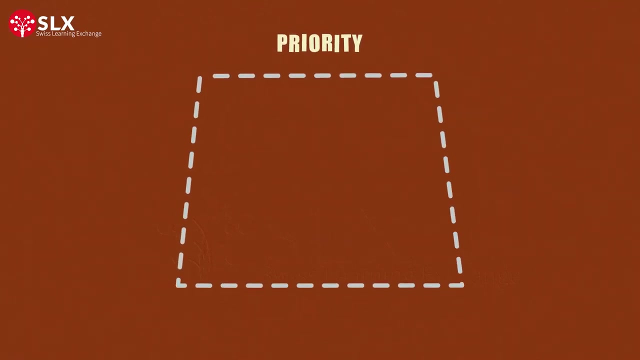 of protecting that area given the available resources. For example, wilderness areas are large regions which are cheaper to protect but have lower biodiversity, whereas biodiversity hotspots are smaller areas which are expensive to protect but have higher biodiversity, higher biodiversity. So if the goal is to conserve a large area inexpensively, you would conserve. 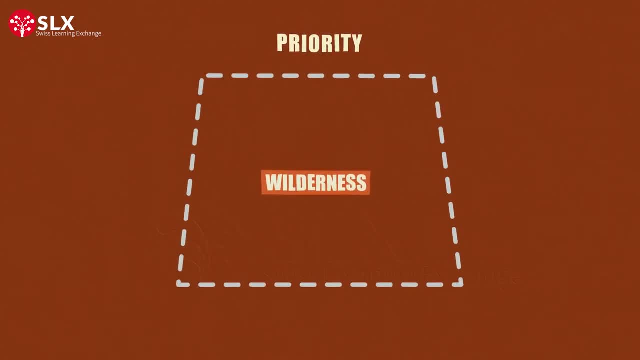 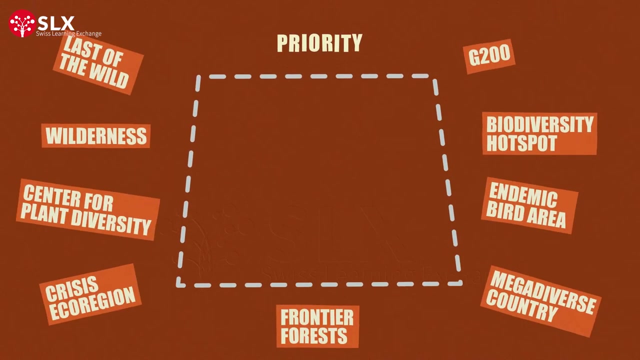 wilderness first, But if the goal is to protect a small area with high species richness, you would conserve biodiversity hotspots first. However, these are only two factors to prioritize protected areas, and there are seven more. This makes prioritization a complicated process of resource. 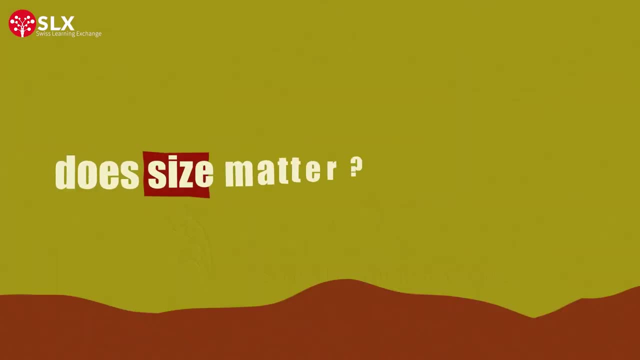 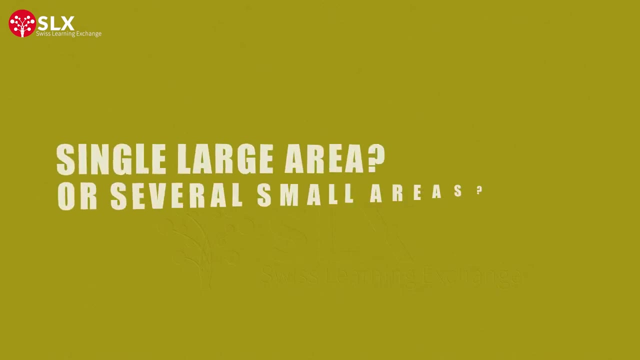 management and impact assessment. Following prioritization, a major challenge will be to identify whether to protect a single large area or several small areas. This problem is often known as the sloss debate among conservationists. There are a multitude of factors that influence the 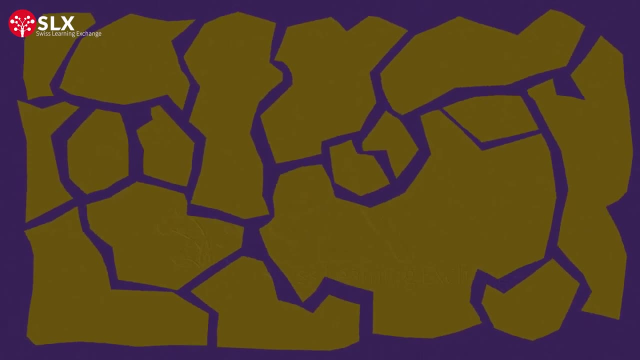 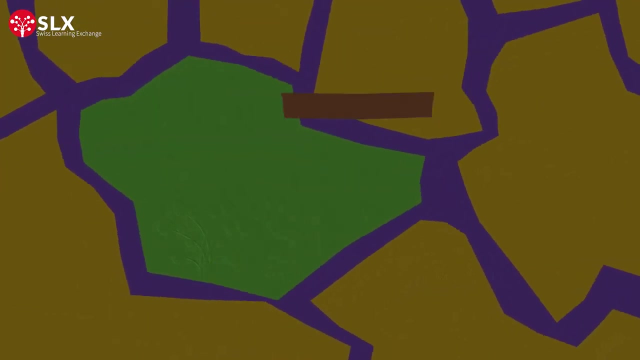 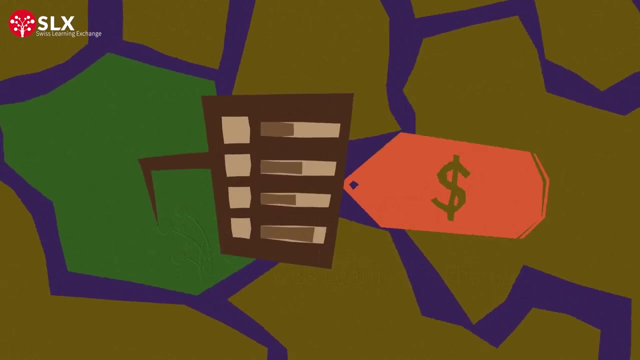 After categorization comes prioritization. Which area to conserve first? To prioritize an area to protect, we must first understand the benefits it provides and assess how vulnerable or irreplaceable the life in the area is. Then we must assess the costs and benefits of protecting that area given the available resources. 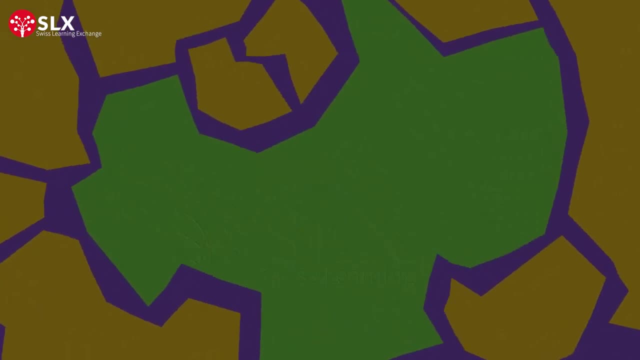 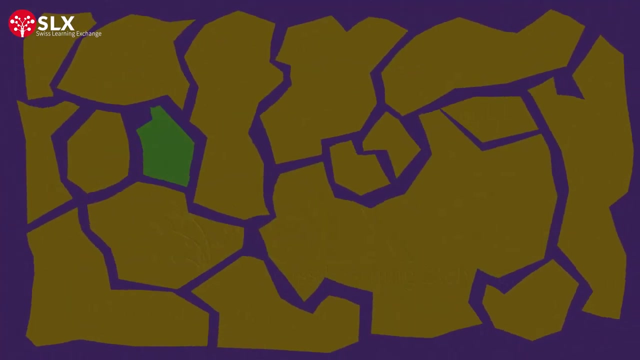 For example, wilderness areas are large regions which are cheaper to protect but have lower biodiversity, whereas biodiversity hotspots are smaller. Category 6 is unique because it allows local people to sustainably extract natural resources. Category 7 is unique because it allows local people to sustainably extract natural resources. 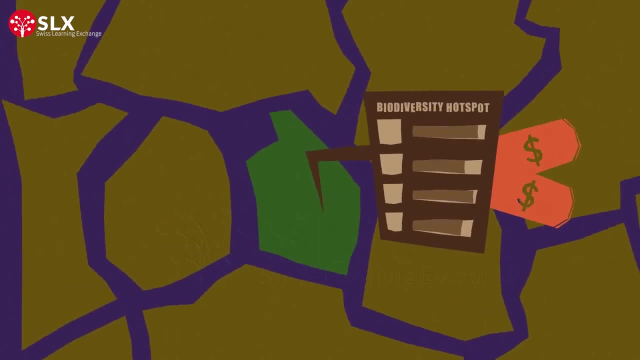 Warranty 3 and 4 are areas that provide the least amount of protection. Which areas to preserve first? To prioritize an area to protect, we must first understand the benefits of protecting that area given the available resources. Smaller areas which are expensive to protect but have higher biodiversity. 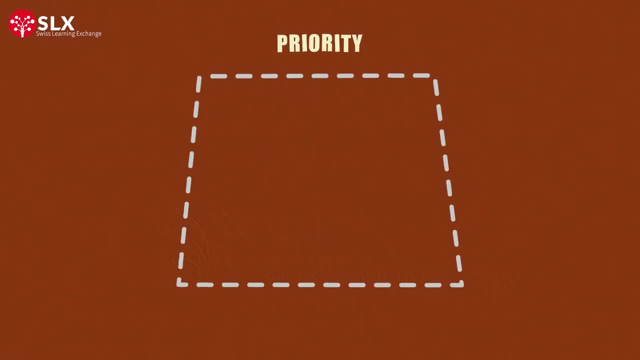 So if the goal is to conserve a large area inexpensively, you would conserve wilderness first, But if the goal is to protect a small area with high species richness, you would conserve biodiversity hotspots first. However, these are only two factors to prioritize protected areas, and there are seven more. 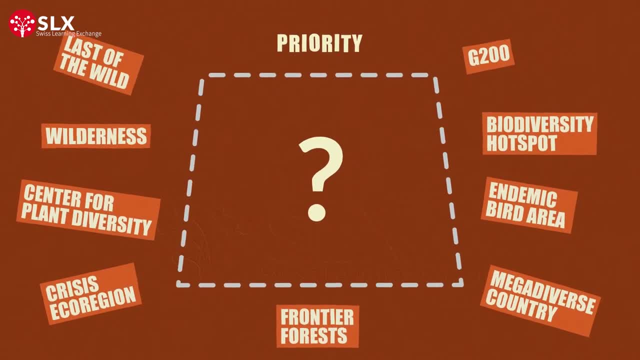 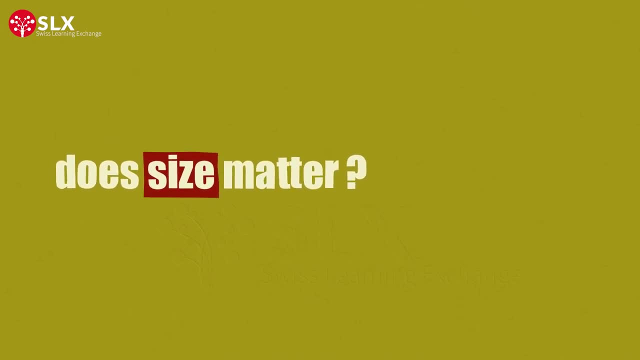 This makes prioritization a complicated process of resource management and impact assessment. Following prioritization, a major challenge will be to identify whether to protect a single large area or several small areas. This problem is often known as the sloss debate among conservationists. 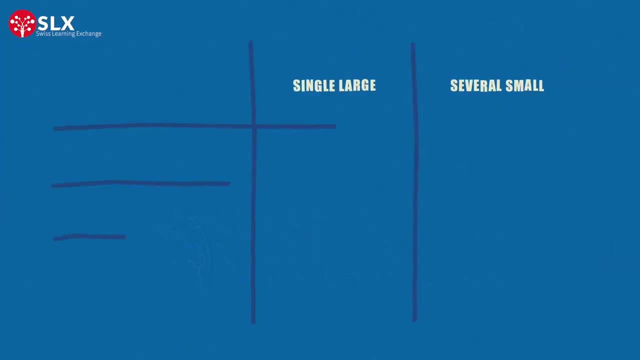 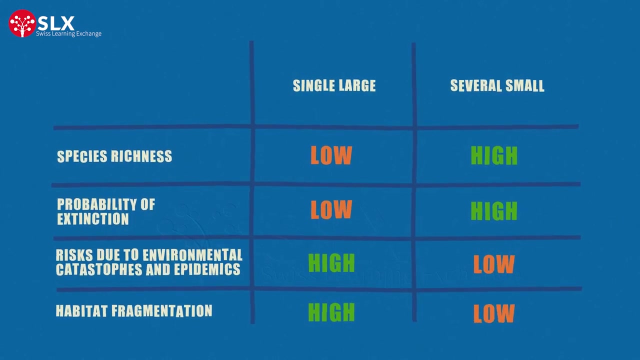 There are a multitude of factors that influence the sloss decision, like species richness, probability of extinction, risks due to environmental catastrophes and epidemics, and the extent of habitat fragmentation As a result, the only thing conservationists now agree on is that there is no clear winner. 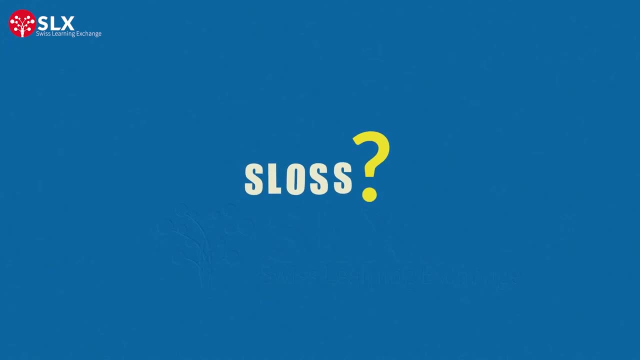 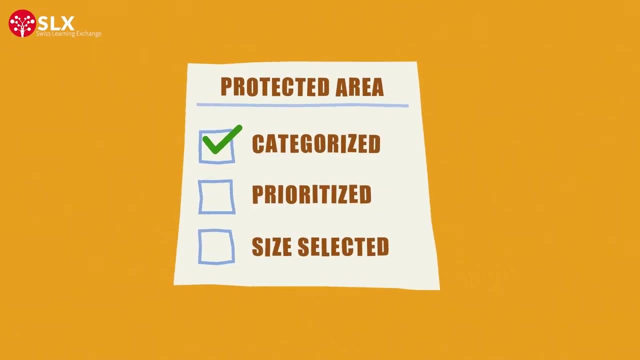 in the sloss debate. Therefore, choosing whether to conserve a single large area or several small areas will be a major challenge. A small area is something each region or country must analyze and decide for itself. Okay, protected area category selected, priority set and area size chosen for conservation. 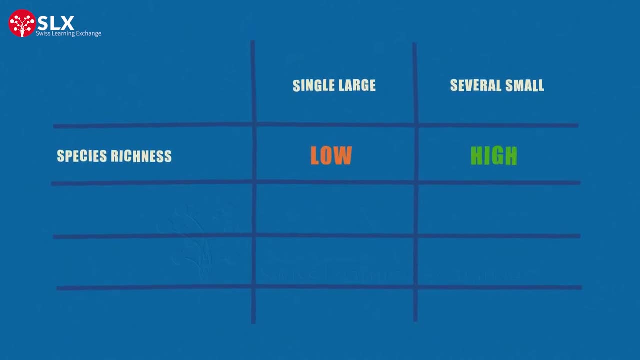 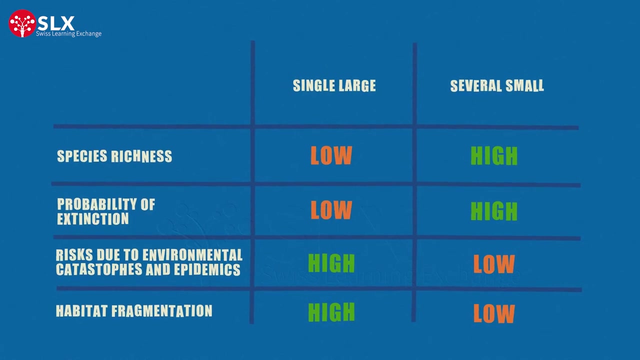 sloss decision. Like species richness, probability of extinction risks due to environmental catastrophes and epidemics, and the extent of habitat fragmentation As a result, the only thing conservationists now agree on is that there is no clear winner in the sloss debate. Therefore, choosing whether to 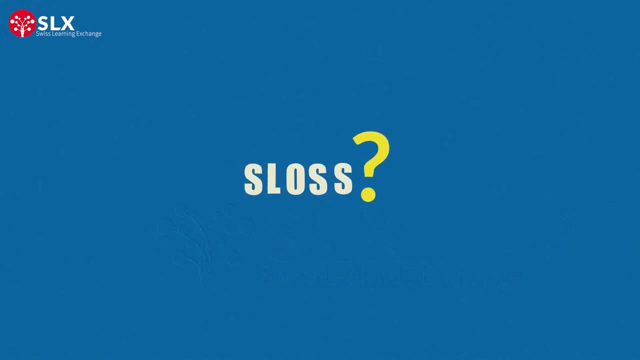 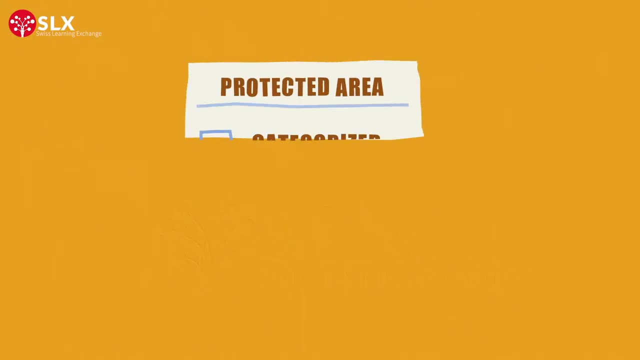 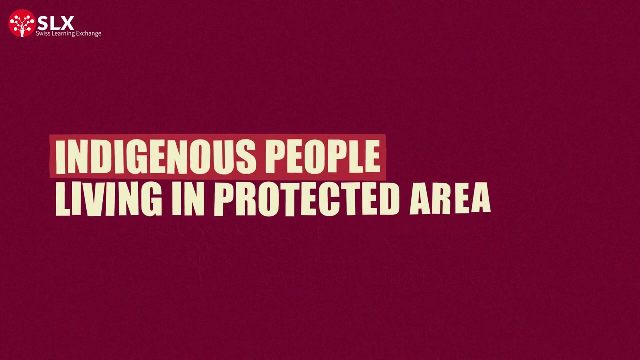 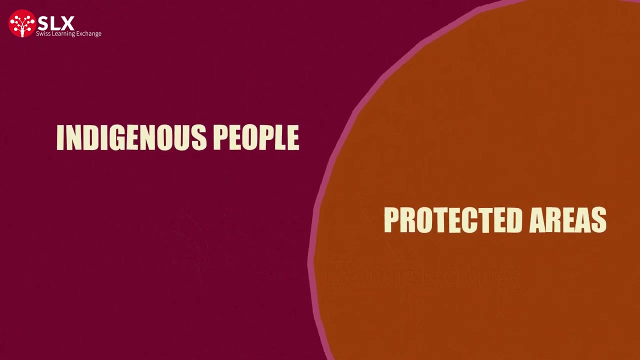 conserve a single large area or several small areas is something each region or country must analyze and evaluate. What happens if My토 find a place where there are loyal and innovative people living in an area with very well? JANLA hemp Sc behöver be be for a certain place. hoch wie sehr Or i optionsb. 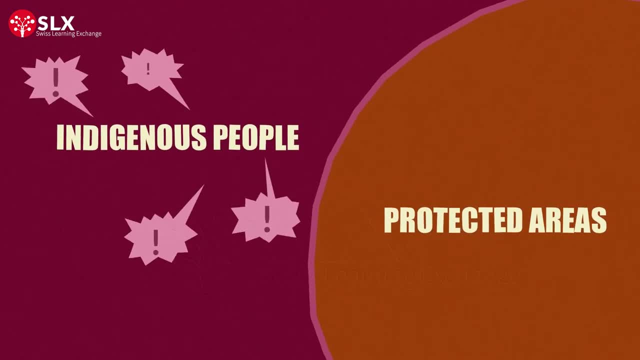 h flower and size of the area chosen for conservation. Are you this person? Historically, indigenous people have been concerned with mainstream conservation and the creation of protected beds. They have repeatedly voiced that these federal actions have consistently been failed, that no place is made up for the development of по셨어요рчив strongerment. This part is the most wonder that we agree on That. the Marine General Act and Dropshifting около 60 killed so many of its people recently- was driven by the government for nameake discovery preparations and 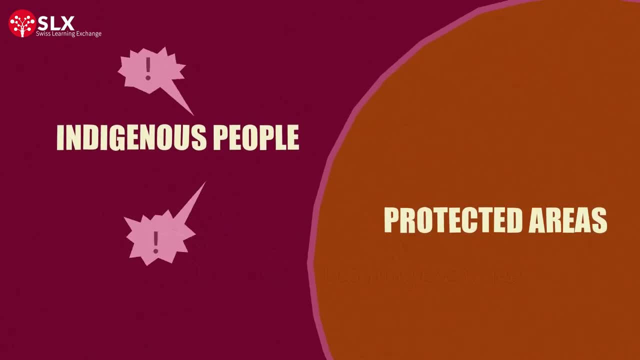 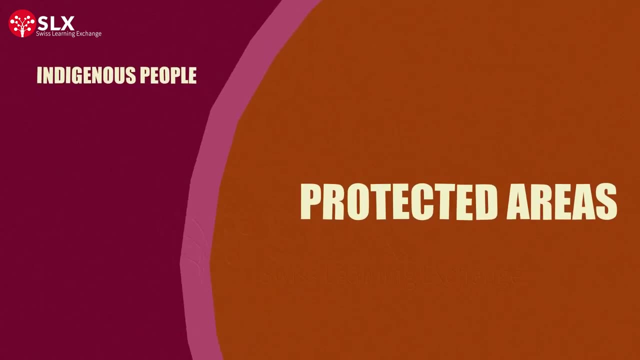 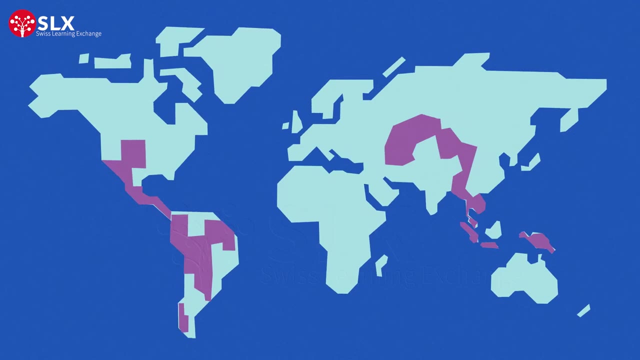 to consider their contributions and their rights when creating conservation areas, which has led to displacement and loss of livelihoods of many indigenous people. In 2019, a report published by the UN revealed that indigenous people live on 20 to 25 percent of the Earth's land surface and are host to most of the world's remaining biodiversity. 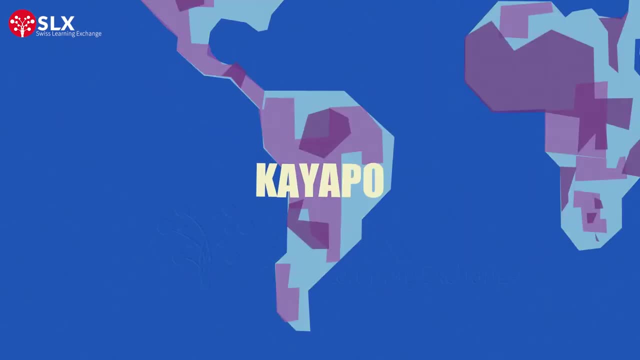 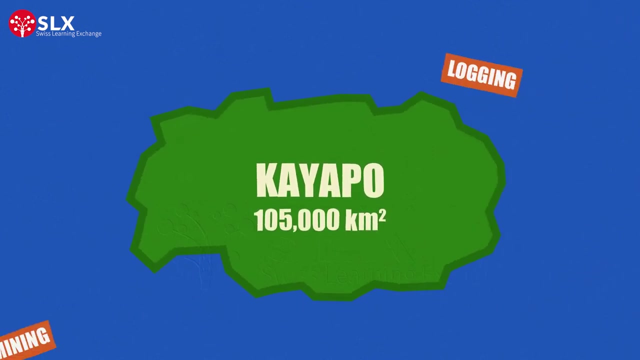 Take the Kayapó people from Amazonian Brazil. They have been able to successfully conserve 105,000 square kilometers of forests in an area that is now plagued by heavy deforestation due to agricultural expansion, logging and illegal gold mining. This shows that indigenous people play a crucial role in conservation. 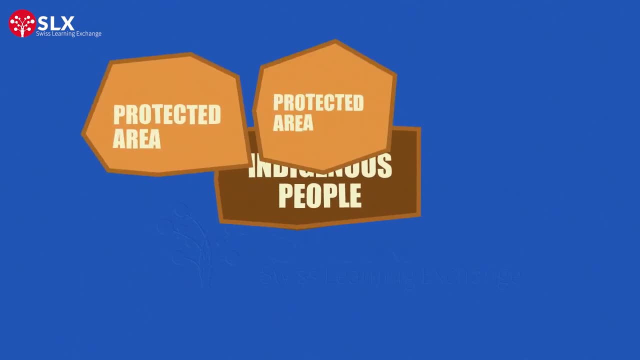 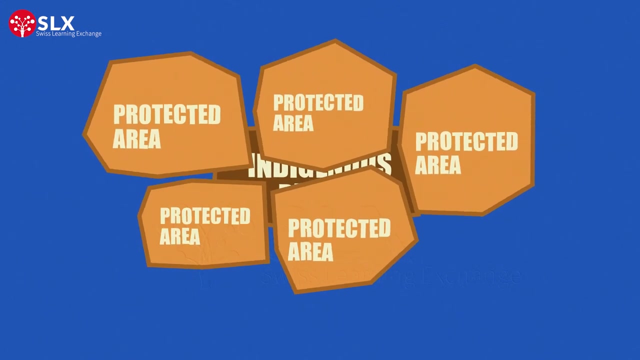 So it is no surprise that 50 percent of protected areas worldwide have been established by indigenous people. This shows that indigenous people play a crucial role in conservation. However, in doing so, many indigenous people have been removed from their ancestral lands in the name of conservation. That's why we need a new approach where the 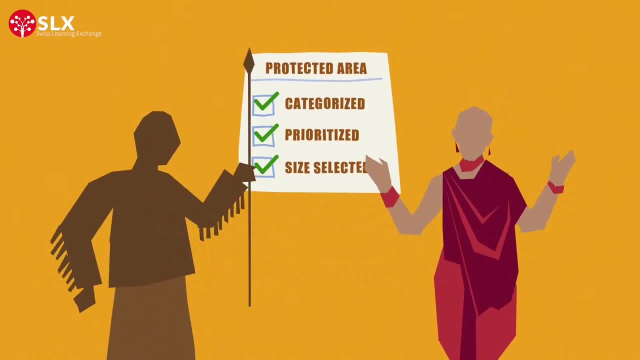 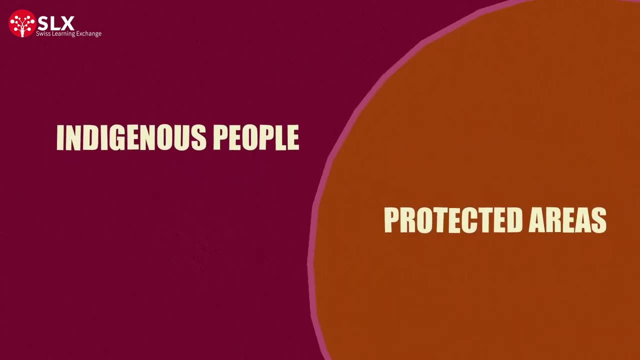 But what happens if you find indigenous people already living in the area? Historically, indigenous people have been concerned with mainstream conservation efforts and the creation of protected areas. They have repeatedly voiced that these efforts have consistently failed to consider their contributions and their rights when creating conservation areas. 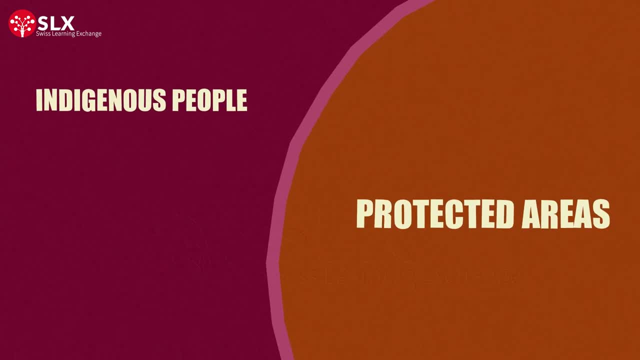 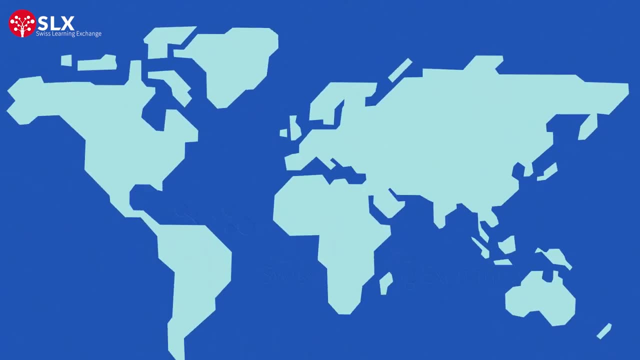 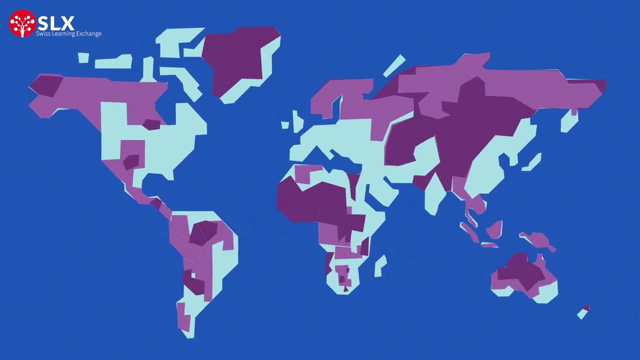 which has led to displacement and loss of livelihoods of many indigenous people. In 2019, a report published by the UN revealed that indigenous people live on 20 to 25% of the Earth's land surface and are host to most of the world's remaining biodiversity. 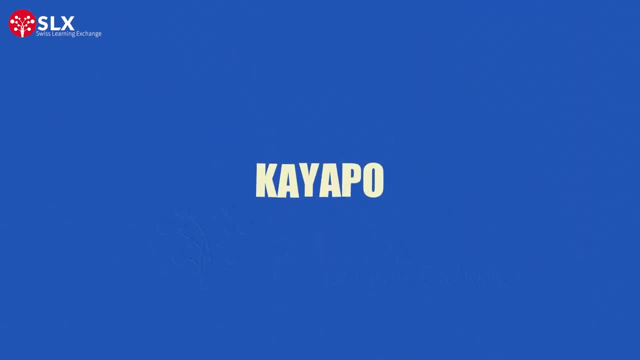 Take the context. They are the Kayapó people from Amazonia in Brazil. They have been able to successfully conserve 105,000 square kilometers of forests in an area that is now plagued by heavy deforestation due to agricultural expansion, logging and illegal gold mining. 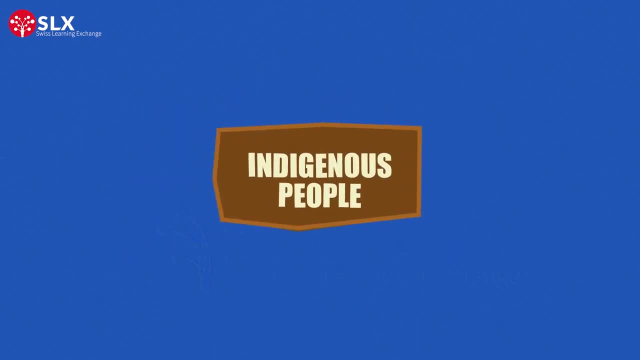 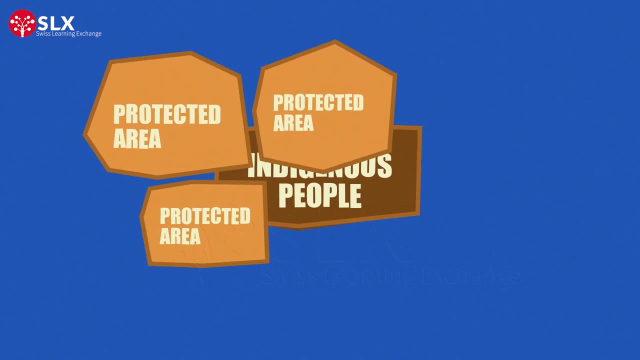 This shows that indigenous people play a crucial role in conservation, So it is no surprise that 50% of protected areas worldwide have been established on traditional territories of indigenous people. However, in doing so, many indigenous people have been removed from their ancestral lands. 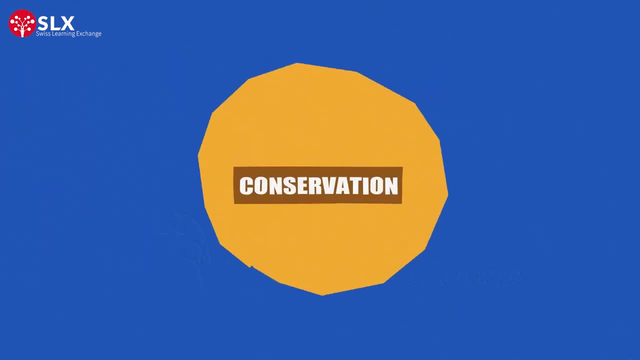 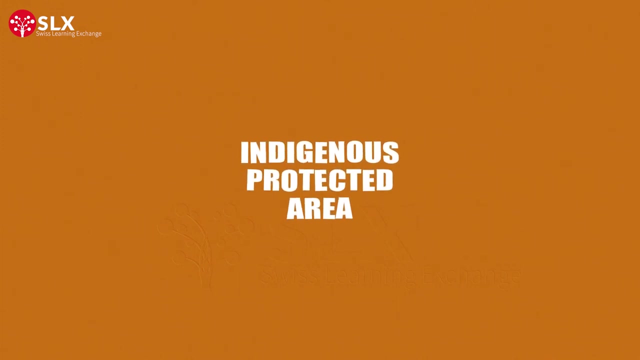 in the name of conservation. That's why we need a new approach where the rights of indigenous people are included as part of effective and equitable conservation of protected areas. Some efforts have been made to make this a reality, For example, through indigenous protected areas and other effective area management. 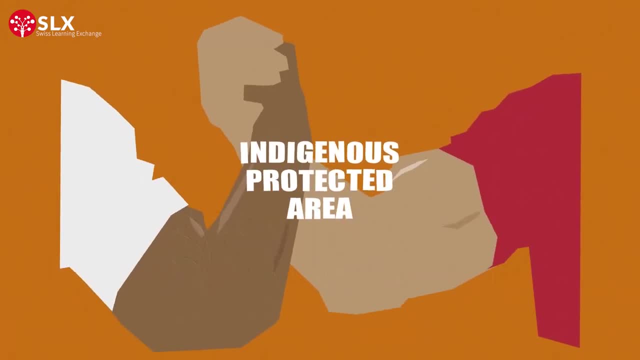 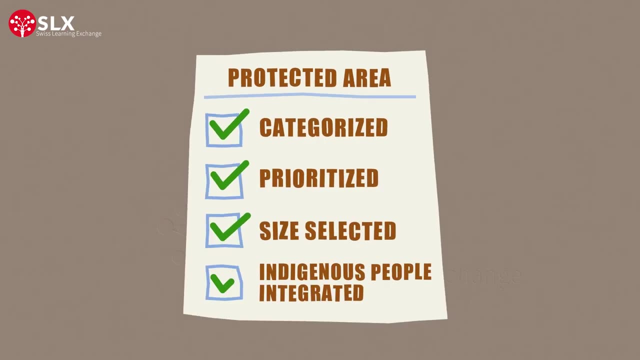 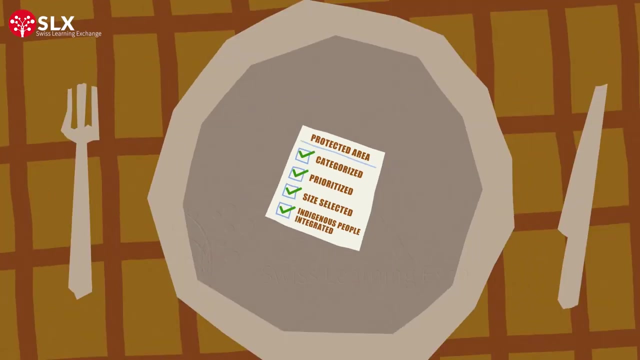 indigenous people are getting involved as stewards for conserving their traditional lands. Even with the successful integration of indigenous people within protected areas, there is one more major complication. What if all that land in protected areas is required for agriculture, so you can feed the population of your country? 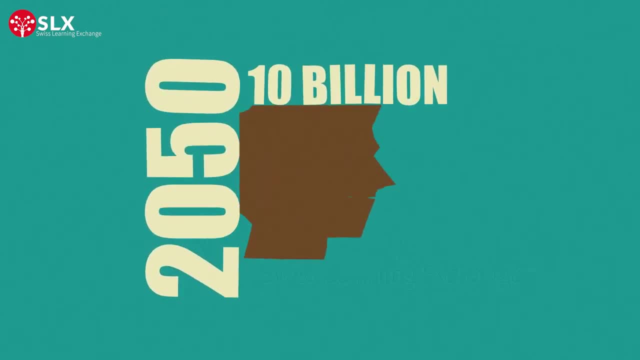 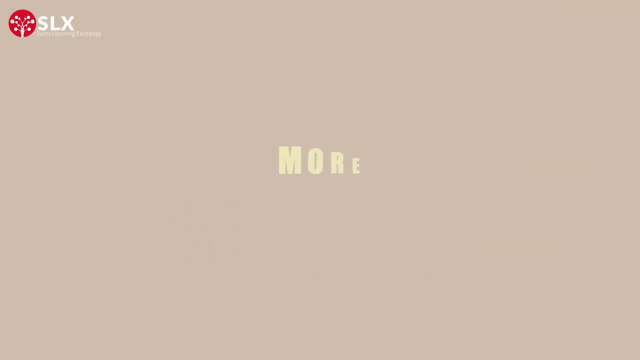 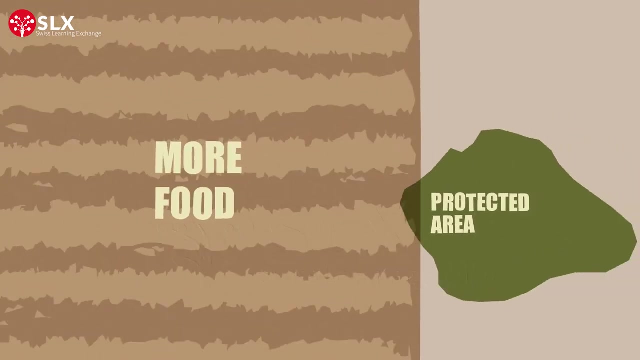 By 2050, there will be nearly 10 billion mouths to feed, which means that food production is going to be a huge challenge. Food production has to increase by 56%. Producing more food requires more land and therefore agricultural expansion would need to encroach on protected areas. 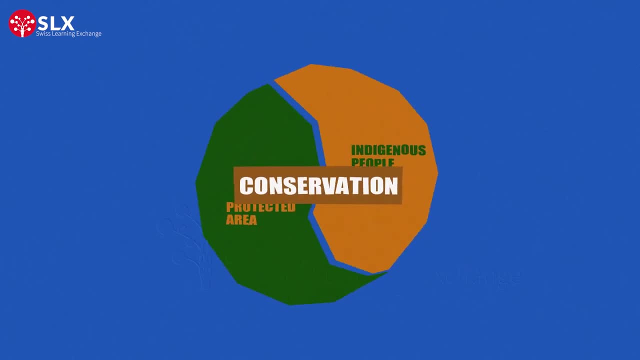 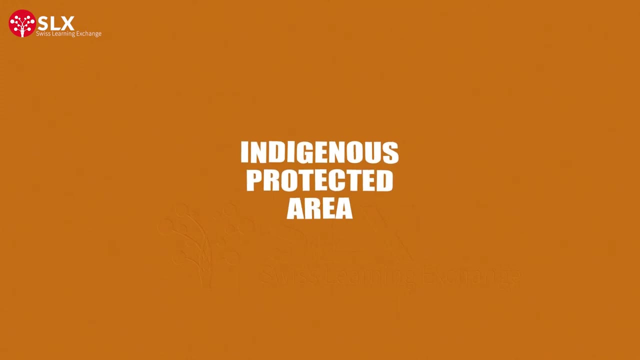 rights of indigenous people are included as part of effective and equitable conservation of protected areas. Some efforts have been made to make this a reality, For example, through indigenous protected areas and other effective areas. indigenous people are getting involved as stewards for conserving their traditional lands. 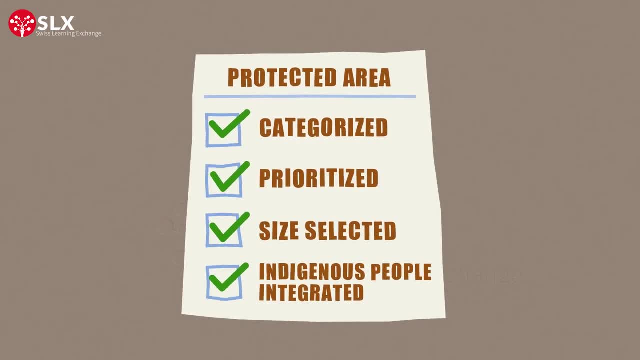 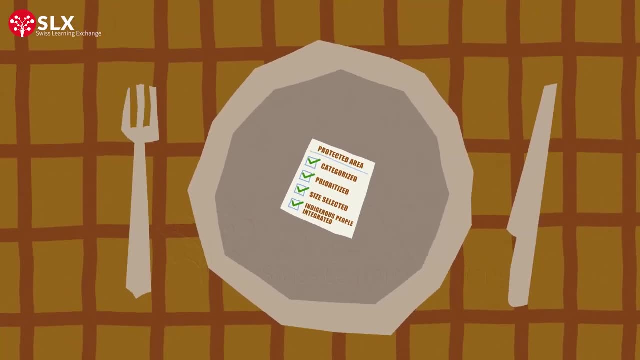 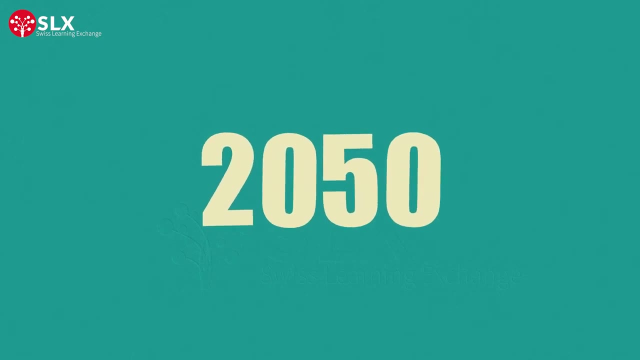 Even with the successful integration of indigenous people within protected areas, there is one more major complication. What if all that land in protected areas is required for agriculture, so you can feed the population of your country? By 2050, there will be nearly 10. 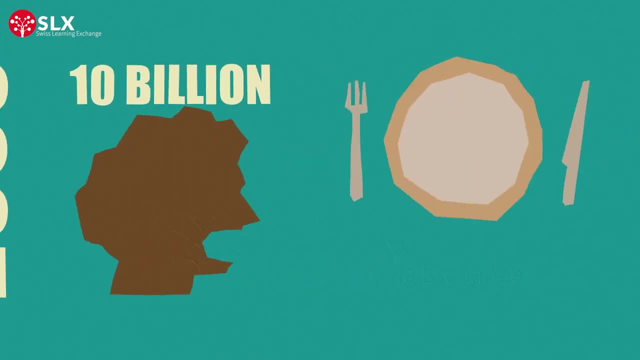 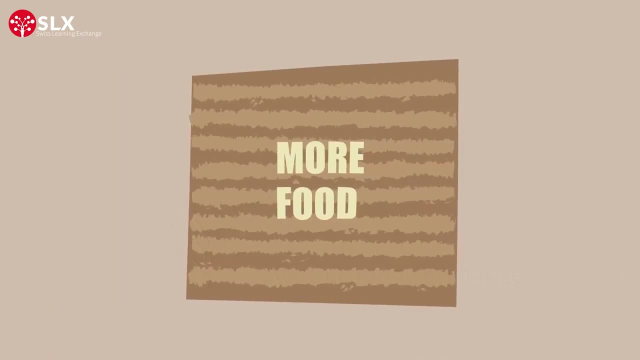 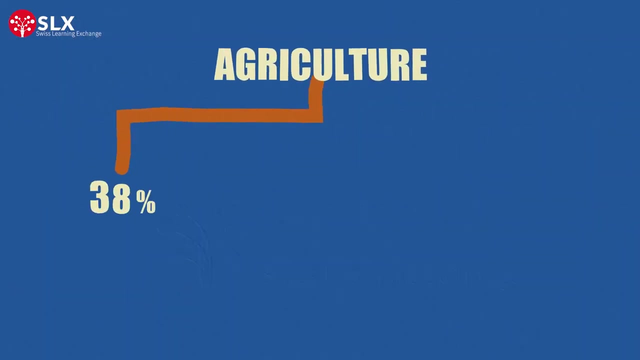 billion mouths to feed. This means that indigenous people will be able to live in protected areas. This means that food production will have to increase to 56 percent. Producing more food requires more land and therefore agricultural expansion would need to encroach on protected areas. Agriculture already occupies 38 percent of the global. 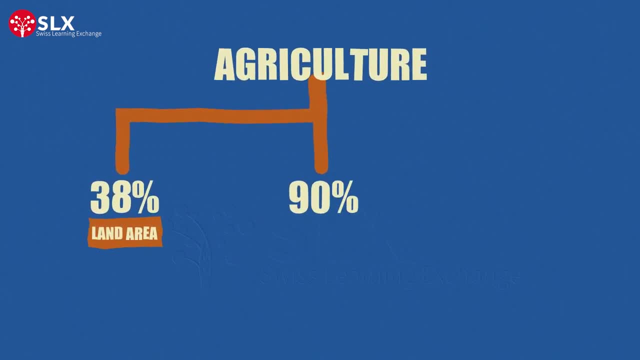 land area today and is responsible for almost 90 percent of the global deforestation, while also threatening the extinction of 52 percent of species on the IUCN's red-hot land ends red list. One solution to this problem is to move away from industrial 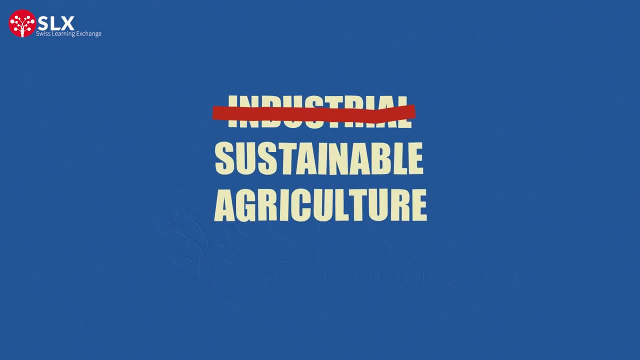 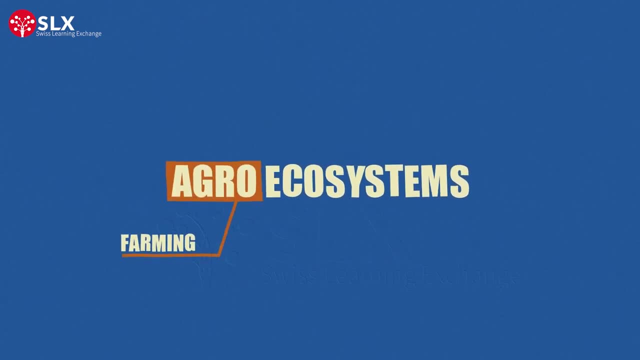 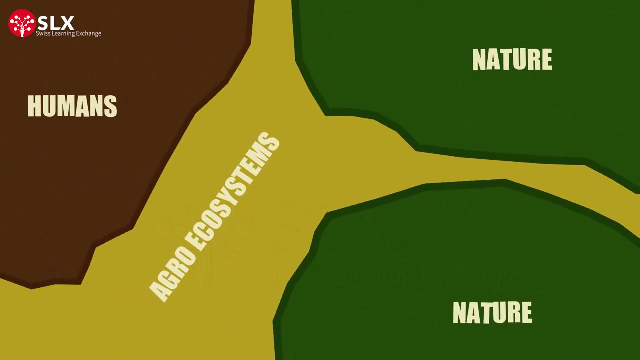 agricultural practices to more sustainable options like agro-ecosystems. These are agricultural practices where traditional farming is integrated with the surrounding natural ecosystems. Agro-ecosystems do not protect or conserve entire natural ecosystems, but they can act as a suitable extension of 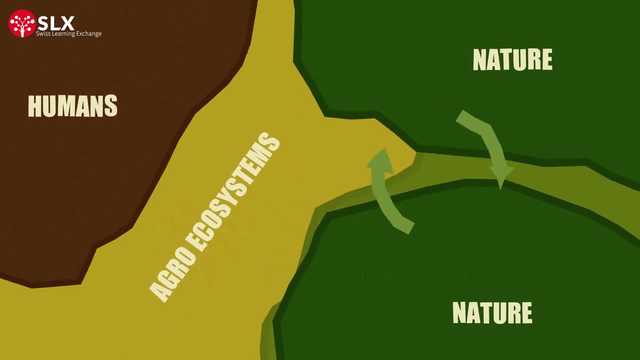 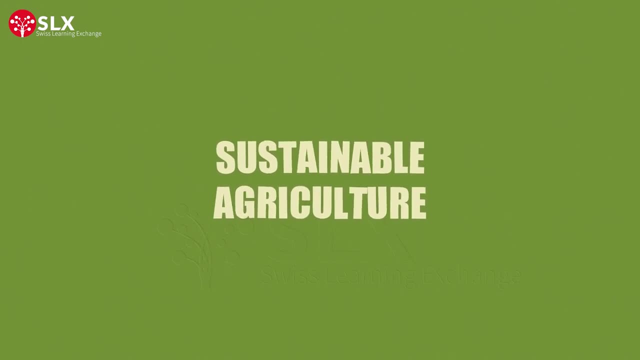 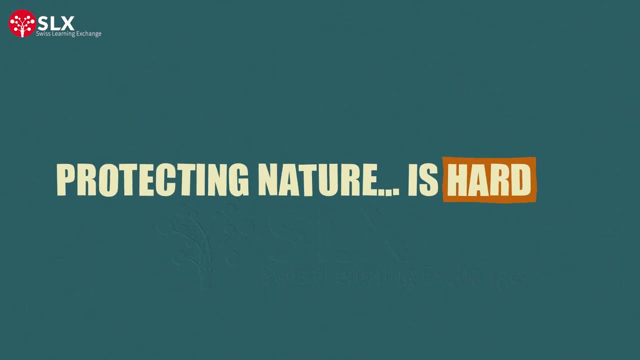 habitats that allow wildlife to move freely between different natural areas. Solutions like these can act as compromises that allow us to feed a growing population and conserve nature. So it turns out that protecting nature is not straightforward. Conservationists all agree that we need to protect 30% of 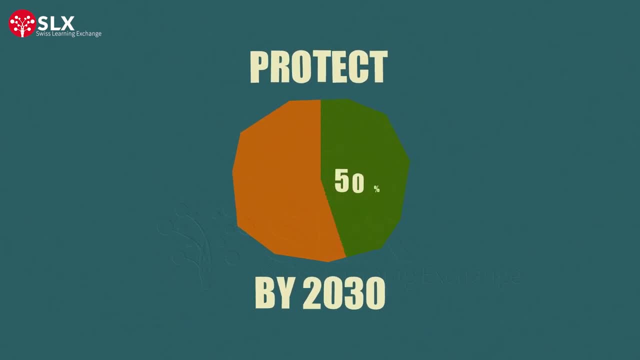 the world's nature by 2030 and 50% by 2050, and we need to protect the environment by 2030.. To prevent environmental, social and economic collapse. However, it's way more complicated than just protect nature, and it's not going to get any easier.